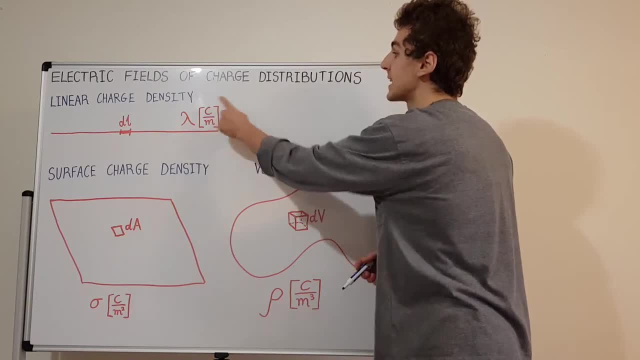 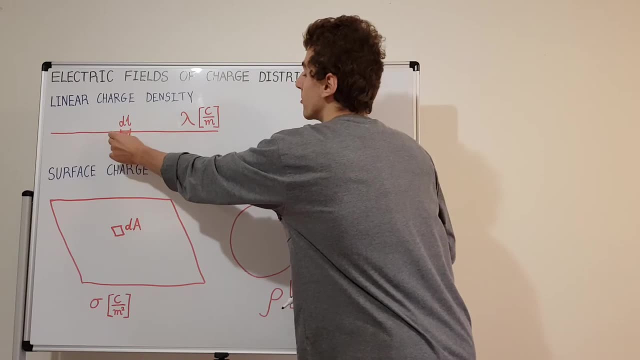 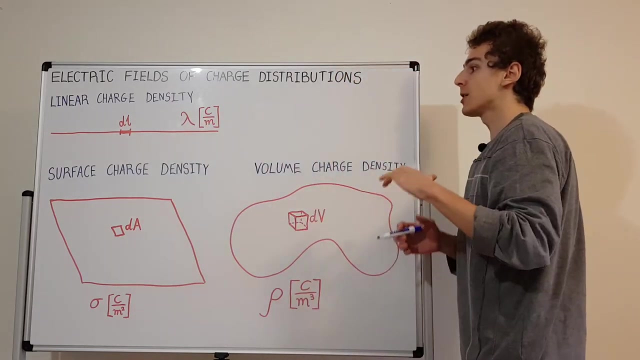 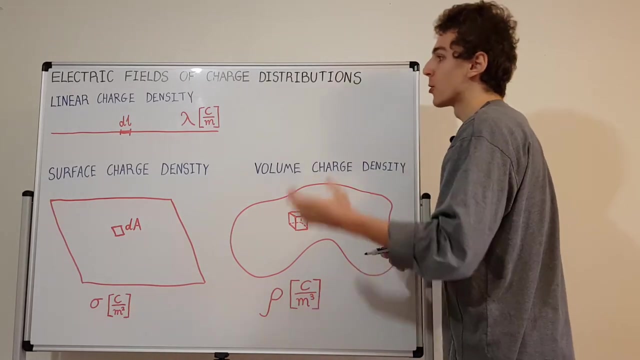 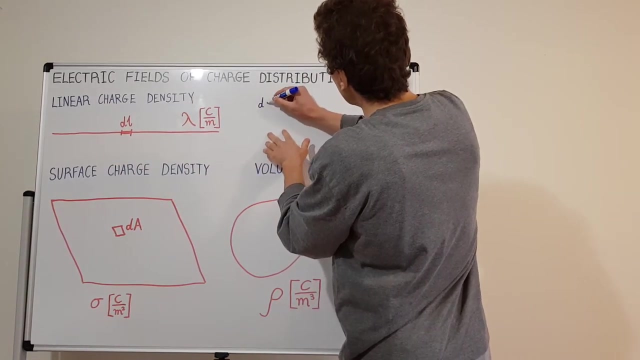 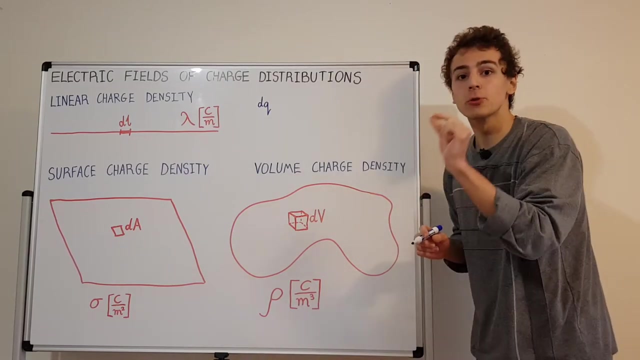 unit length, So that's coulomb per meter. These are the SI units for linear charge density. So what is a little chunk, A little chunk DL going to look like? Well, it's going to be a tiny, infinitesimal slice of this line. And so what you can actually do to calculate how the electric field would change is you need to calculate how the charge is distributed. So what is the charge going to be? Well, the charge you can also break up as a little dq. So what we could do is we could have a tiny little dq, So that's dq. This is a lowercase q And that is an infinitesimal little chunk of charge. 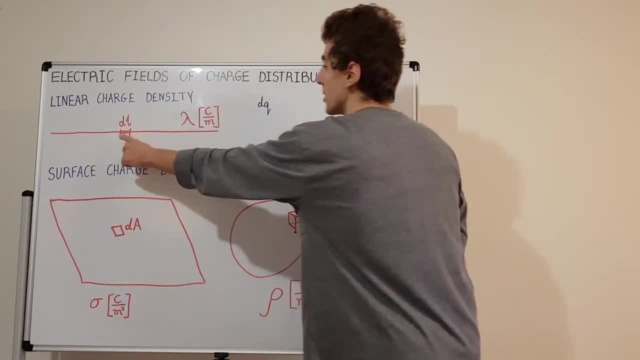 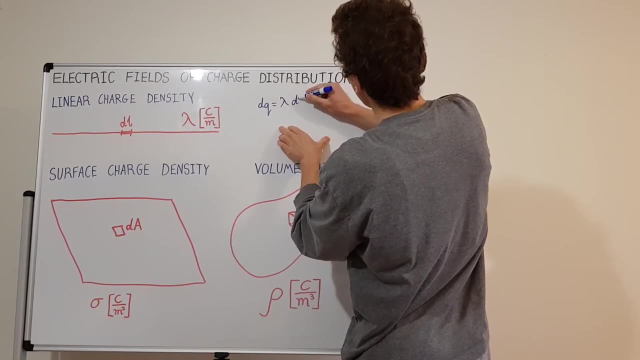 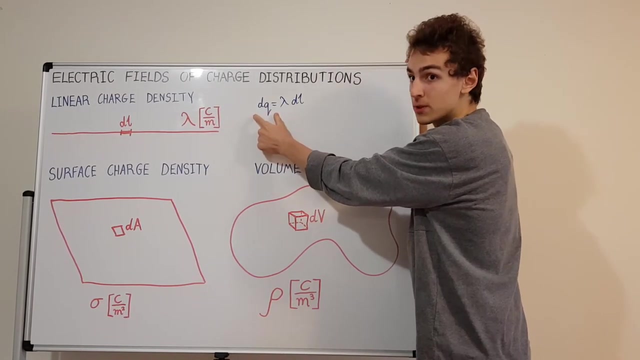 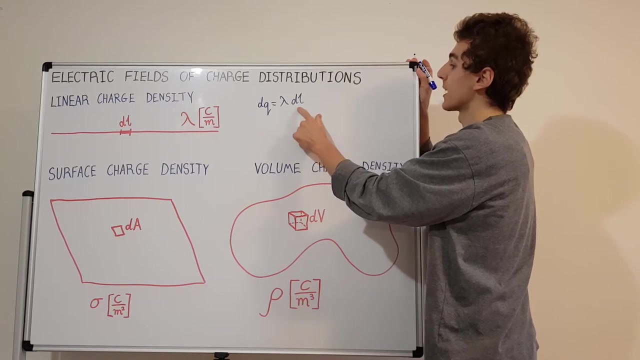 And what is the dq going to be in this situation? Well, it's actually going to be the linear charge density lambda times DL. Let's see if the units match up. This has the unit of charge. This is in coulombs in SI units. This over here is coulombs per meter, or charge per unit length, And this has units of length. This is in meters. So the units of length are going to cancel and you're just going to be left with coulombs. 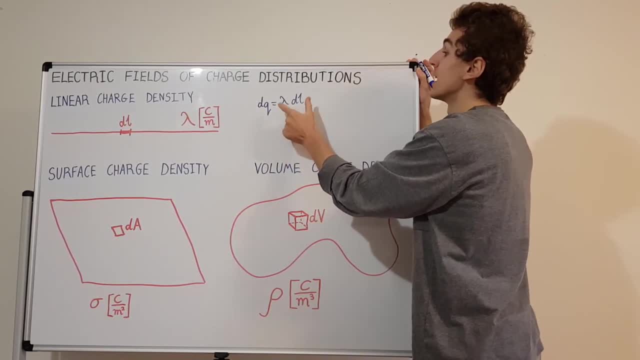 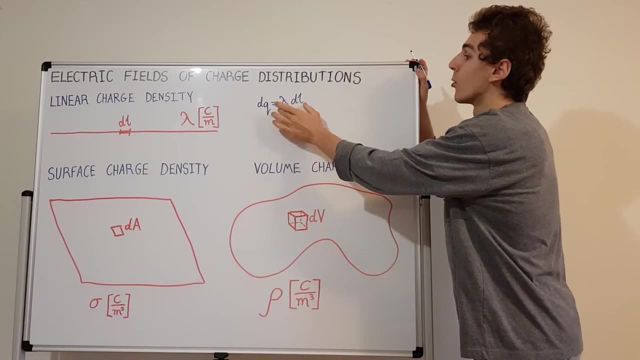 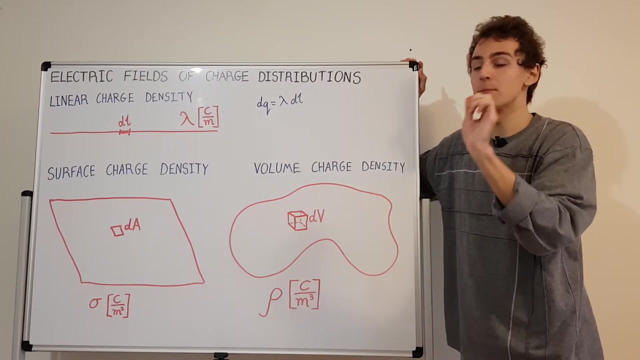 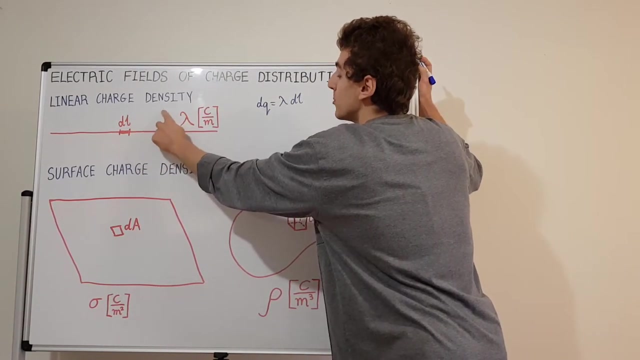 So this is actually the amount of charge that would lie in every little chunk over here. So then, if you wanted to calculate the electric field, you would integrate all of these little charges and you would also take into consideration their distance from a point. So electric field is always calculated at a point. So if you're looking at some location up here, at some point over here, there would be a distance R from that DL, and you would take that distance, you would square it, you'd go 1 over R squared. 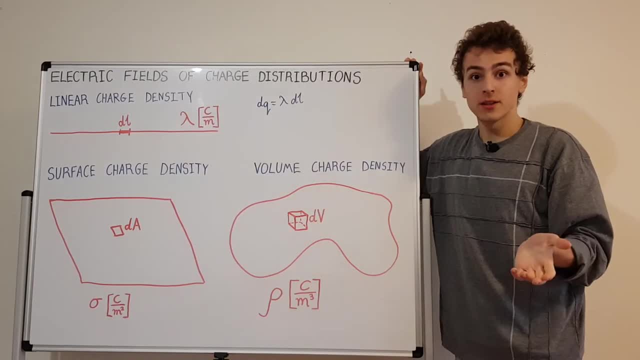 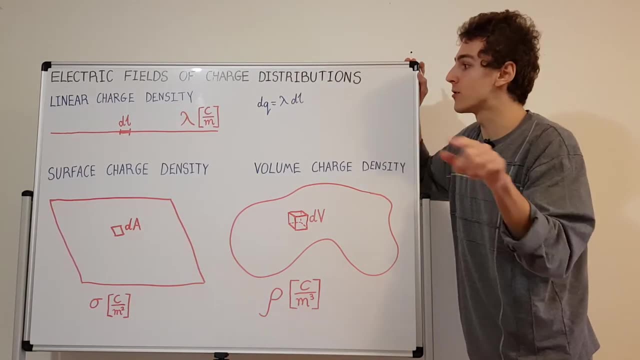 Why 1 over R squared? Well, it's because we know that point charges- point charges- behave in accordance to coulombs law. So coulombs law for force tells you that there's a 1 over R squared relationship, And if you're looking for electric fields, you just remove one of those charges from coulombs. 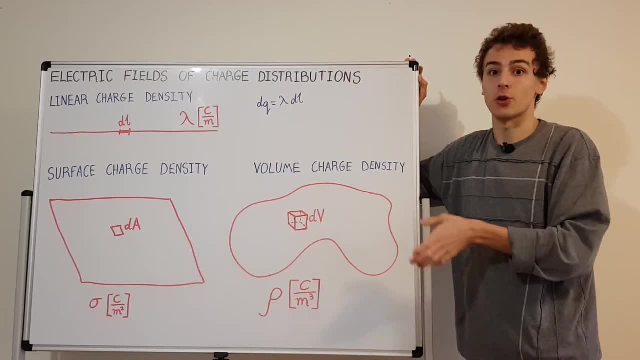 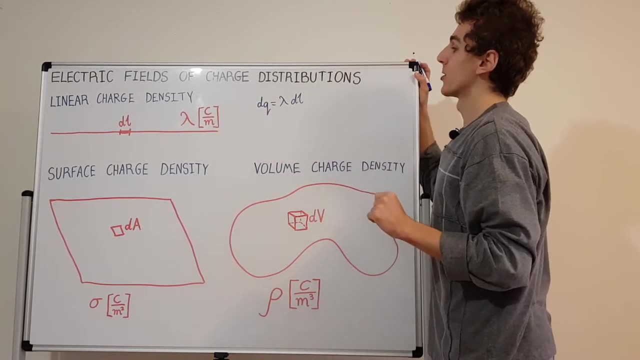 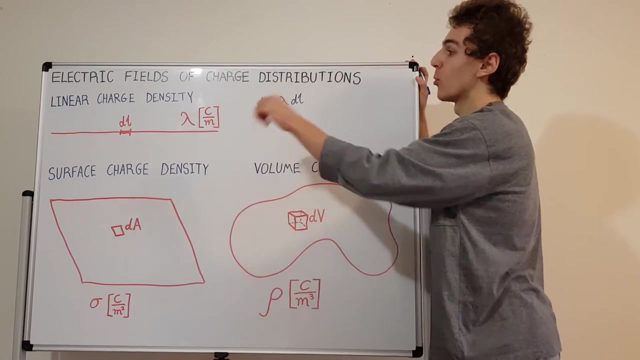 law, because you're just interested in the force per unit charge. That's what the electric field is concerned with. So this is our first step to working out something that has a linear charge density. What if it's not on a straight line, Or it doesn't actually have to be straight? it could be some kind of one dimensional line. 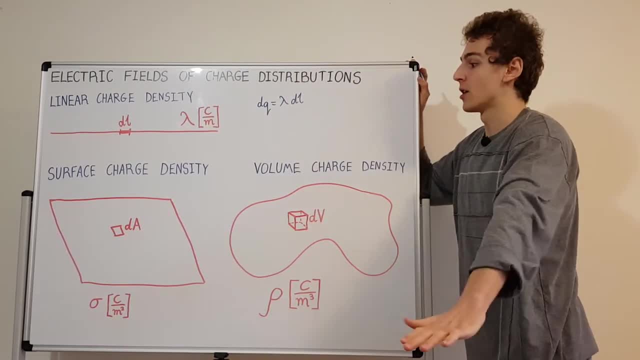 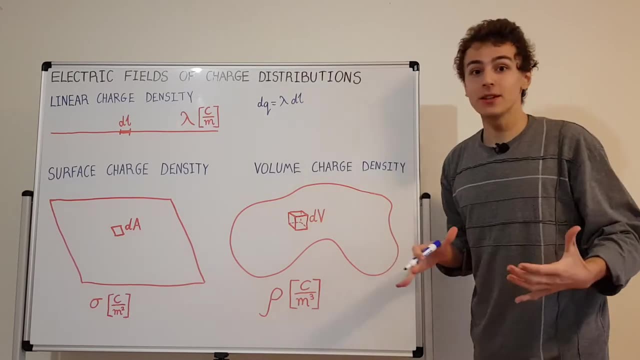 What if it's not on a one dimensional line? What if it's on a surface? What if all of these little chunks of charge are distributed evenly on a surface? Or what if it's not even an even distribution? What if there's some variation? 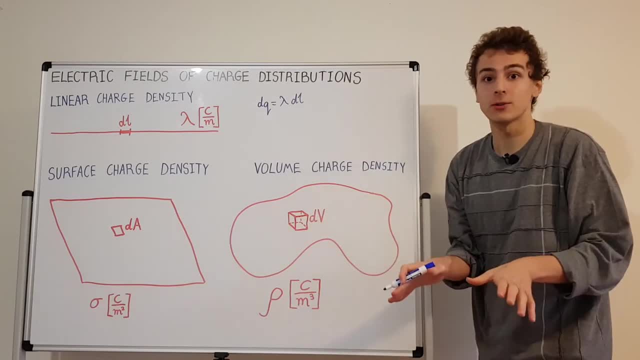 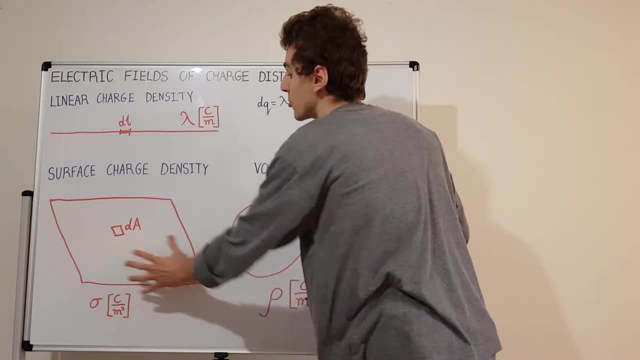 What if there's a lot of charge near the middle and not a lot of charge on the outside? How would we deal with that kind of electrostatics problem? Well, we'd have a look at surface charge density And that's this situation over here. 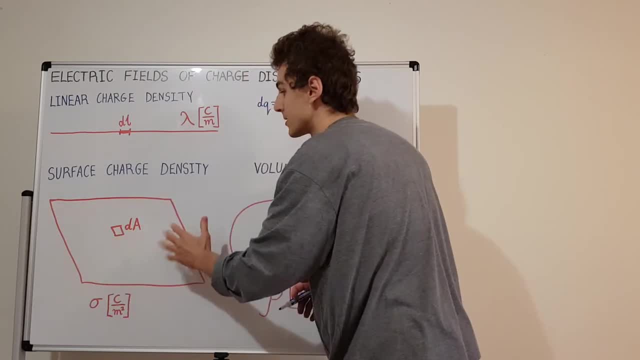 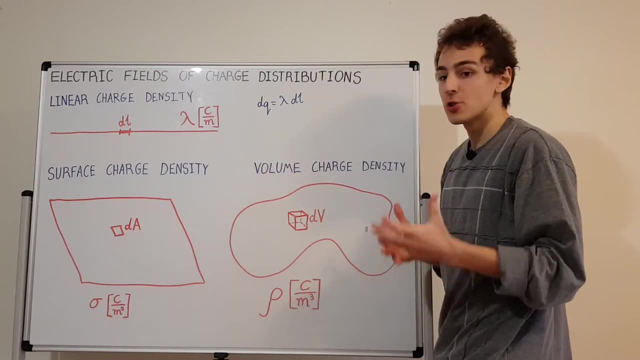 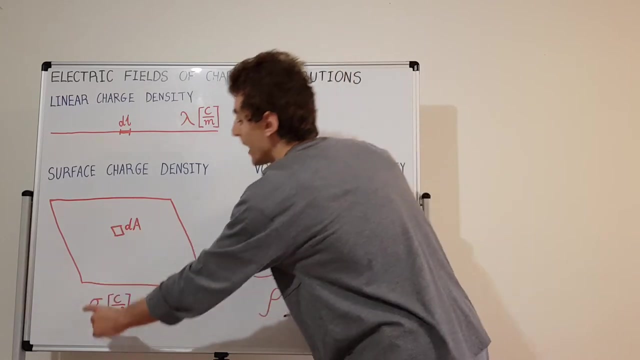 So imagine we have some kind of surface- This is any two dimensional surface- It has some kind of charge distribution. How would we quantify that distribution? Well, we would use the surface charge density, And that's represented by the Greek letter sigma. So over here we have lambda, that's the linear charge density, and now we have sigma, the. 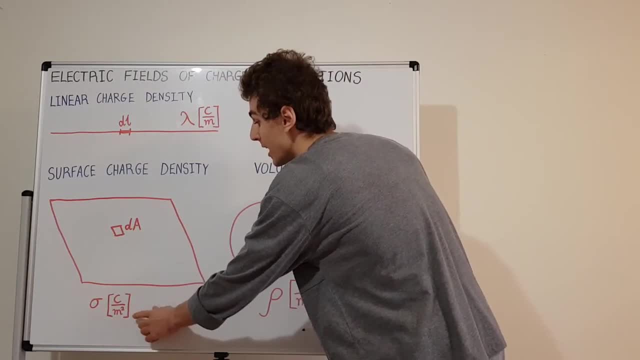 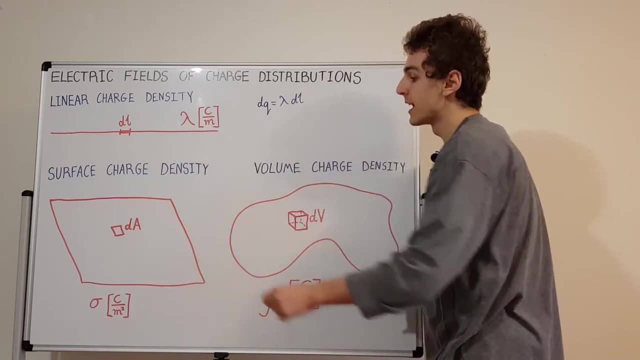 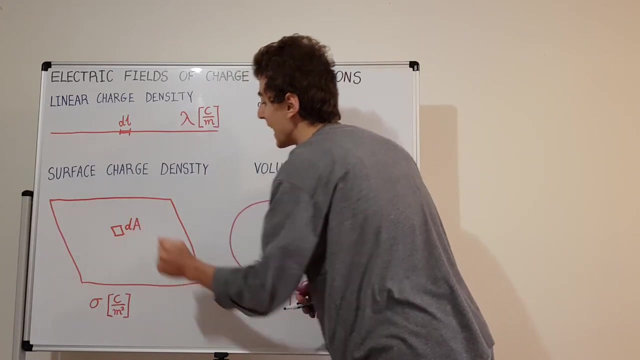 surface charge density The units are different. Here we have coulomb per meter squared, So this is charge per unit area. Over here we had charge per unit length. now we have charge per unit area. So what we're interested in is a tiny, infinitesimal area which we can call dA. 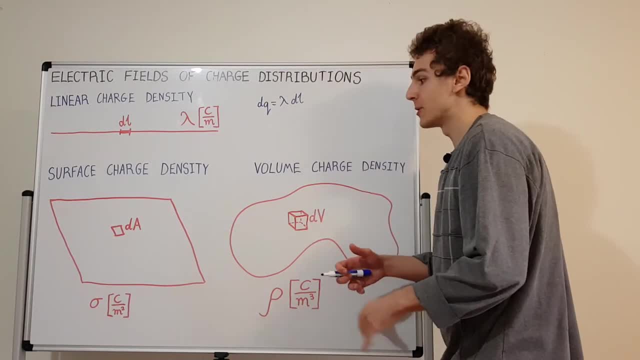 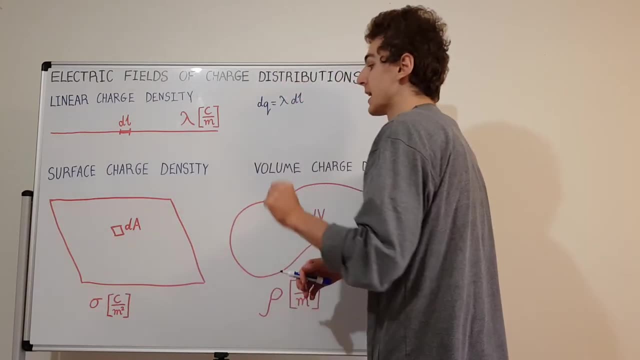 Sometimes this is called dS for a surface. if you're doing a surface integral- because what you will actually end up having to do is an integral over this surface, But you're going to take each of the charges in each of the tiny little chunks dA. 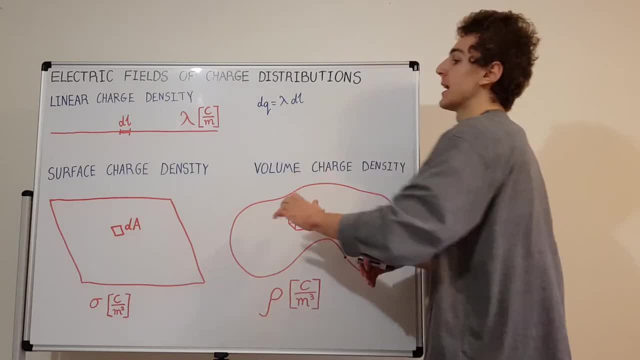 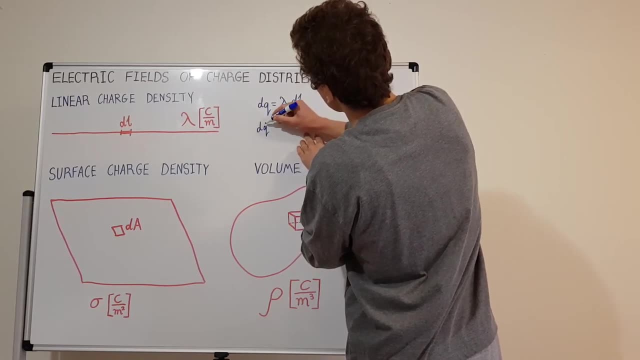 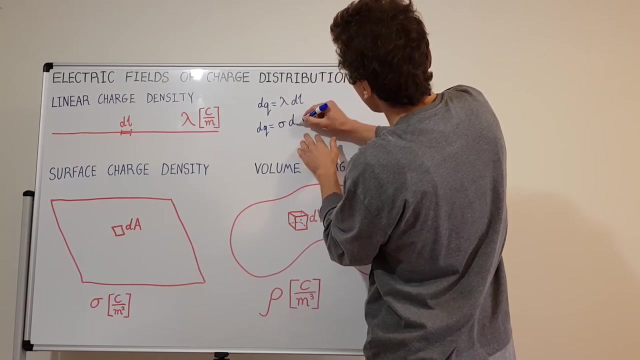 So how would a little chunk of charge, how would it look like in the surface charge density case? Well, we would have something like dQ. This is a tiny little dQ That's going to be equal to sigma times. dA right. 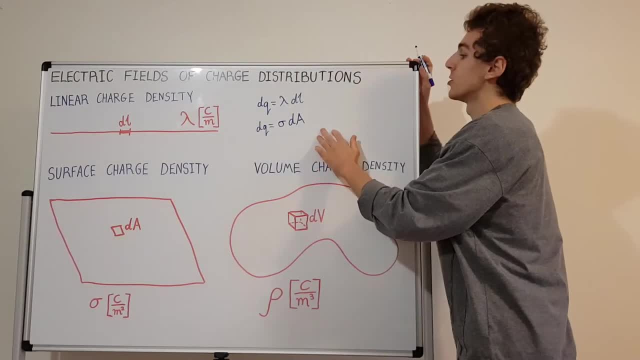 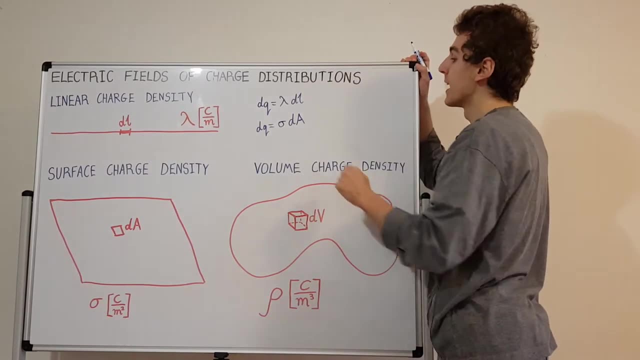 Sigma times dA. Make that A a little bit better. There we go. So this is a tiny, tiny little chunk of area. You can think of it as dx by dy if it's Cartesian coordinates, And this over here is the surface charge density. 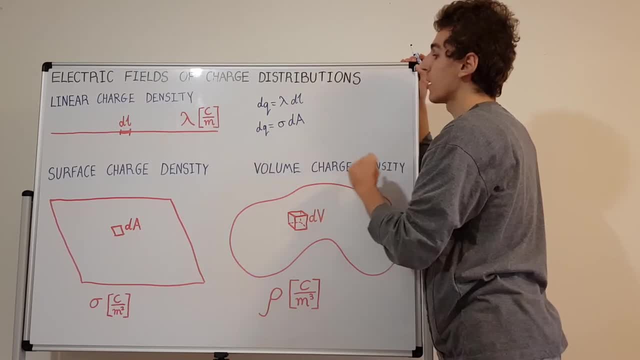 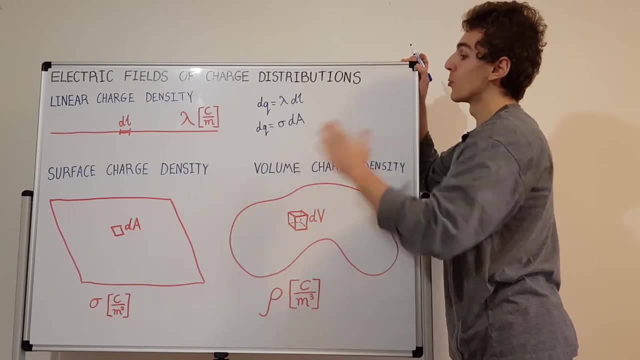 That's the charge per unit area. So again the units work out. Here we have units of charge, Here we have charge per area multiplied by area. So the units of area, which in SI units is meters squared, they're going to cancel out. 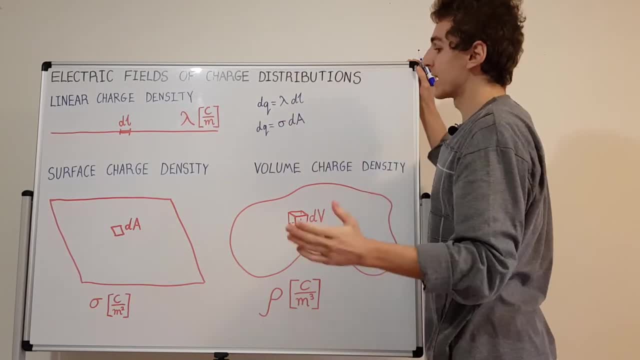 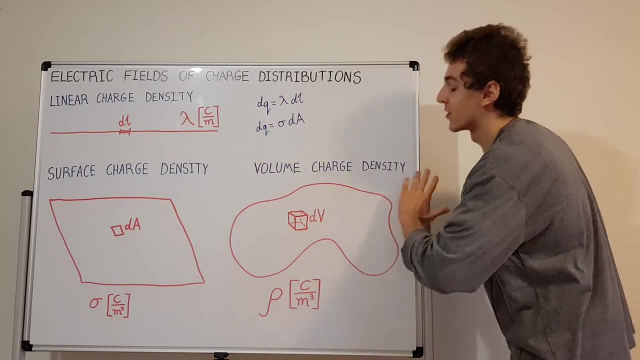 And so we'll be left with coulombs or units of charge. Now let's have a look at something that is an extra dimension. So we've had one dimension, two dimensions, and now we're going to have a three-dimensional system, and that is volume, right. 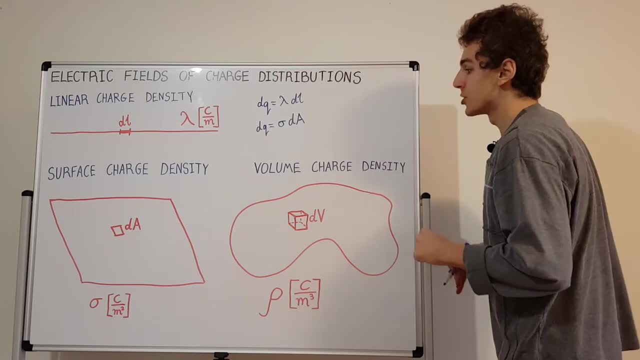 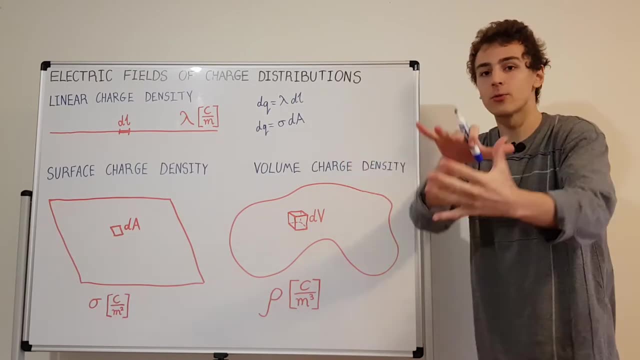 Volume charge density is our next quantity of interest. So volume charge density- Volume charge density is useful if you have a three-dimensional charge distribution. So there's charge everywhere in 3D space and each point in 3D space has a value associated. 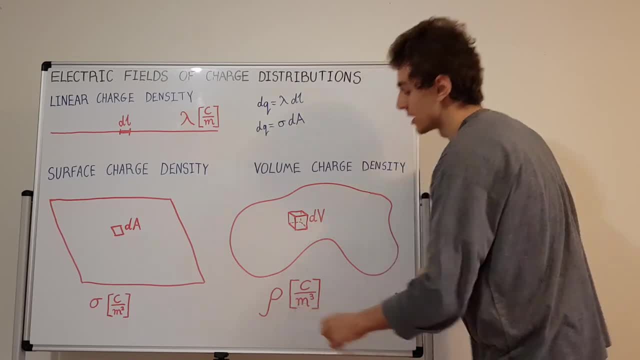 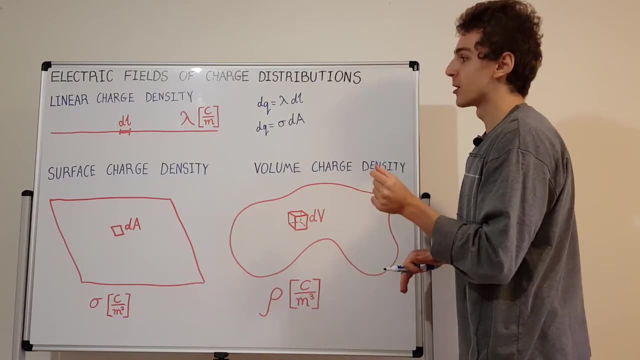 with it, So rho. the Greek letter rho is used to denote volume charge density. Now, in the previous two examples we also had this little infinitesimal. What is the infinitesimal in the volume charge density case? Well, it's dv. 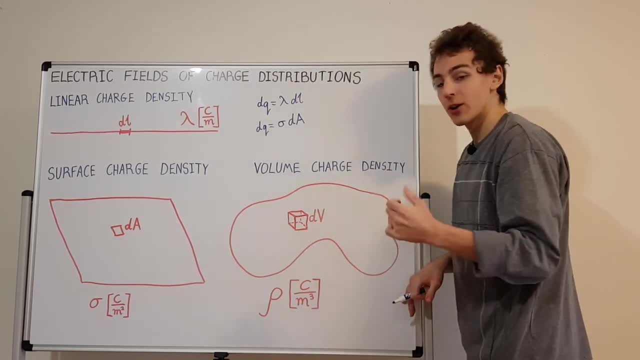 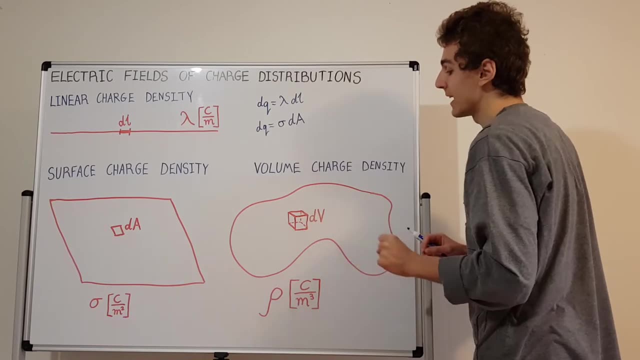 And I've drawn a little cube to illustrate dv. So in Cartesian coordinates This would be dx dy dz. So dx dy dz is a tiny, tiny little cube in 3D space, And when we're doing the integrals for all of these, we're going to take the limit as 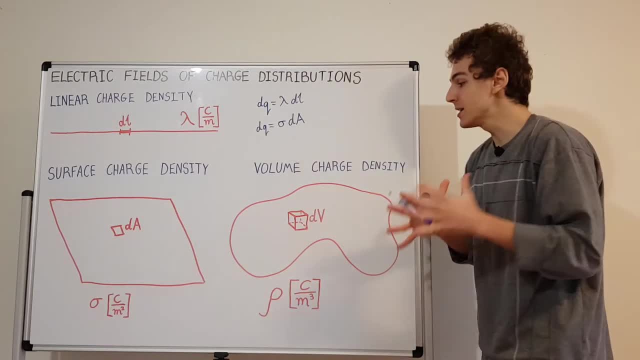 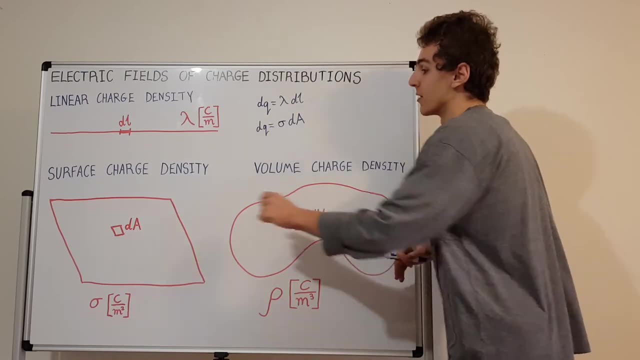 these infinitesimals go to zero, right? An integral is essentially a sum with some limits, And the limits state that this guy has to go to zero, this guy has to go to zero and this guy has to go to zero. So they're never actually equal to zero. we just take the limit as they approach zero. 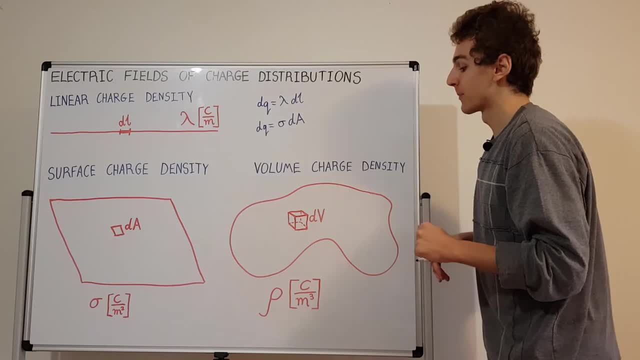 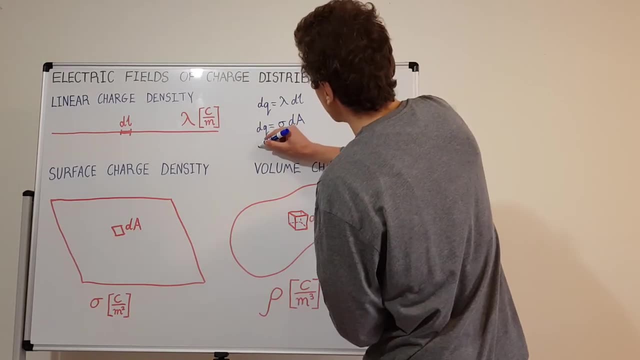 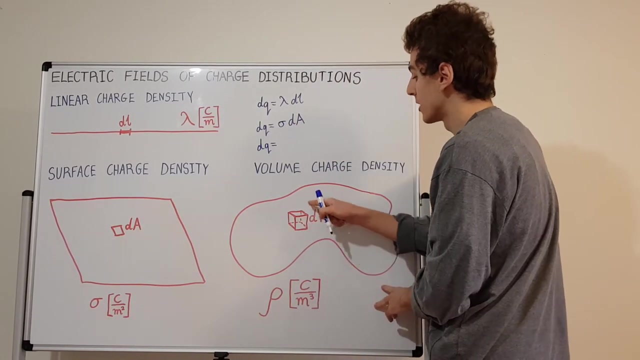 and we see what value we get from our integral. So how would a tiny chunk of charge look like in this scenario? Well, we've seen the pattern so far. So dq would be equal to a tiny little increment of charge, or a tiny little chunk of charge. 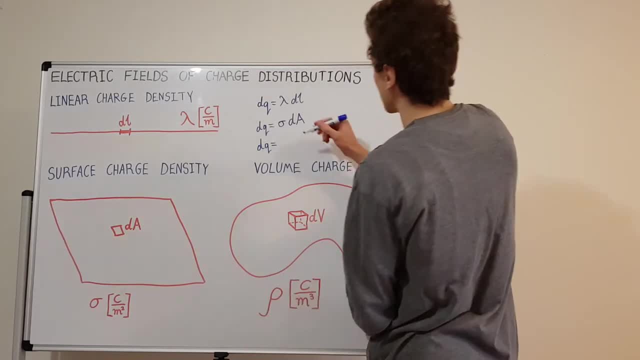 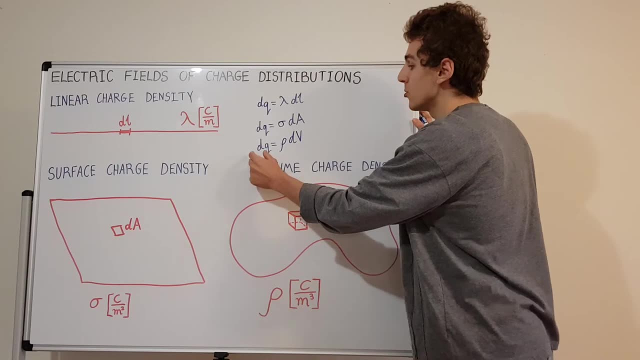 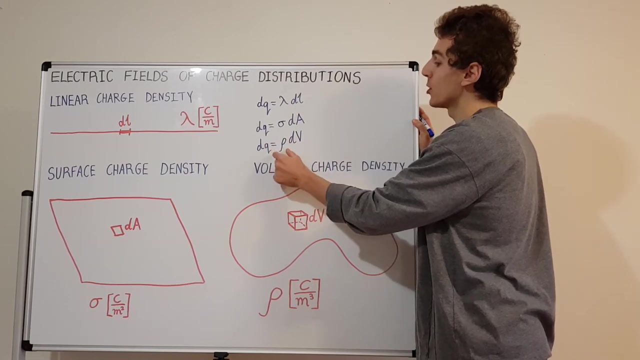 which is going to be a tiny volume, times the density. So it's going to be rho dv And let's check the units again. So dq, That's units of charge. This is charge per unit volume and this is volume. So volume and we have per unit volume. those guys are going to cancel out and we'll be. 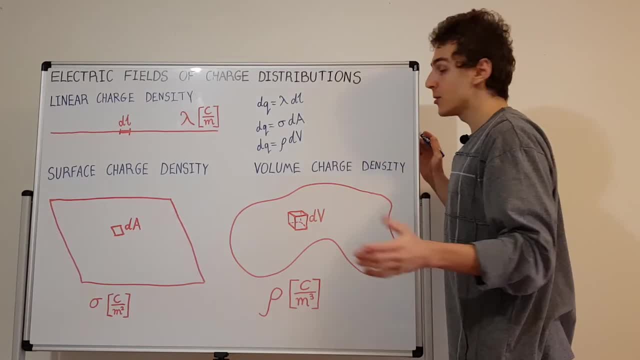 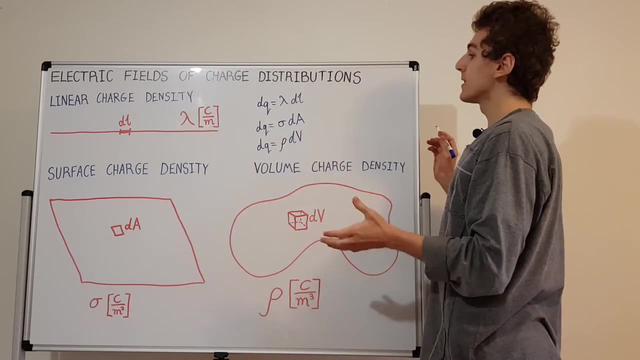 just left with units of charge And si units. both of these sides are going to be coulombs, so we'll have coulombs on both sides. So then, what we would do is we would actually take each of these tiny little chunks and 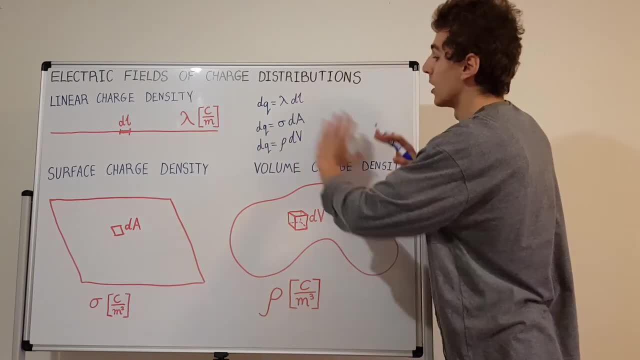 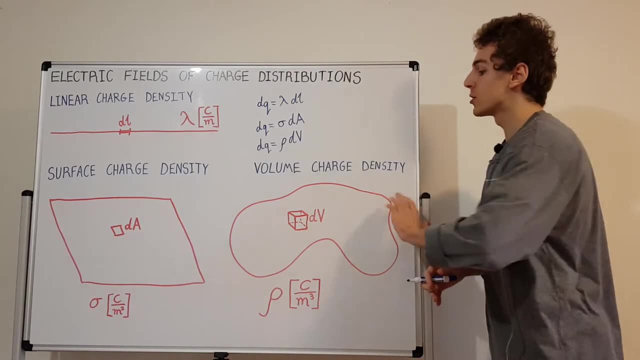 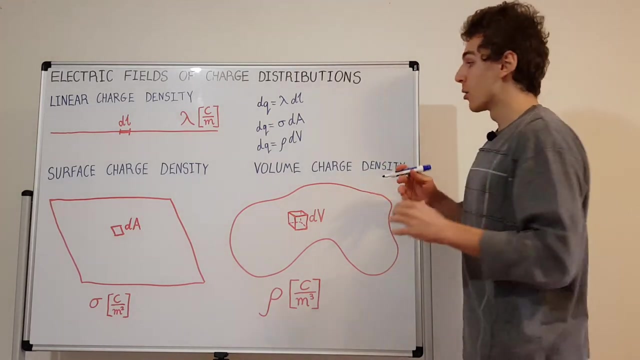 we would integrate them with respect to all of over the entire domain. right? So the domain, The domain could be a line, the domain could be a surface or the domain could be a volume in three-dimensional space In general, in 3D space. if you want the total charge, what you would do is you would go. 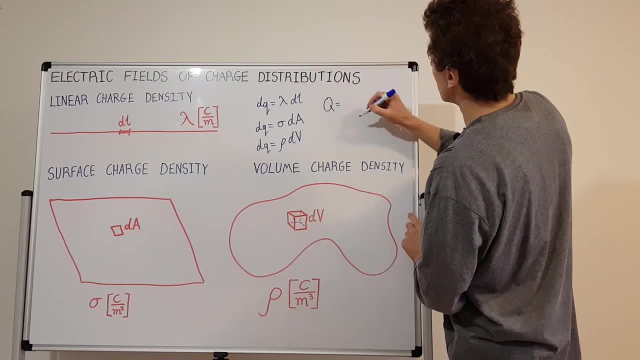 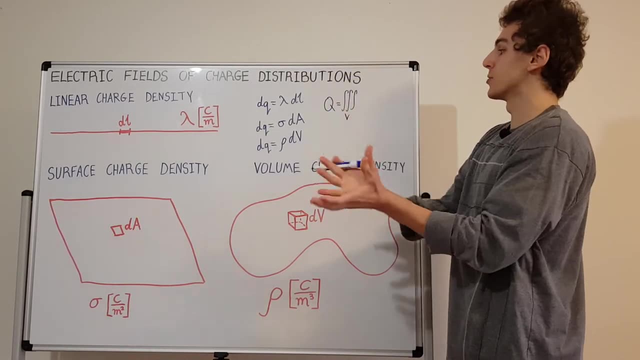 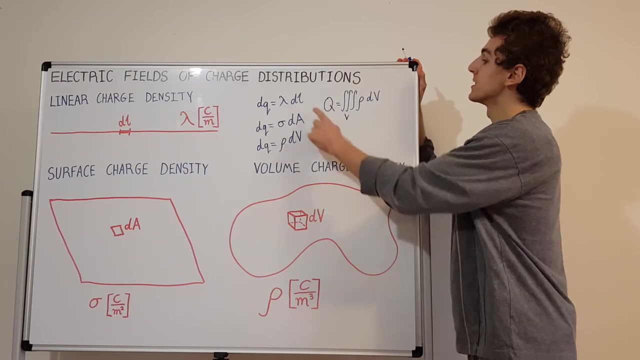 q. the total charge is equal to the volume integral. So we need three integral signs over the volume. This is some kind of volume that's enclosed by a surface: times, rho, dv, right. This over here is the total volume. This over here is the total charge from a 3D scenario where there's a three-dimensional 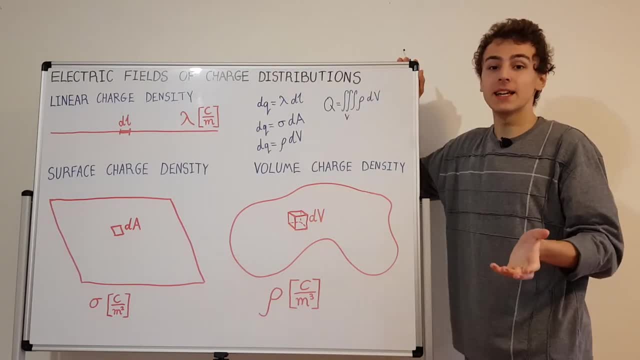 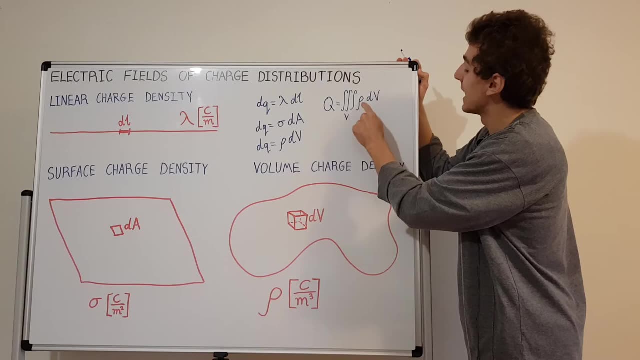 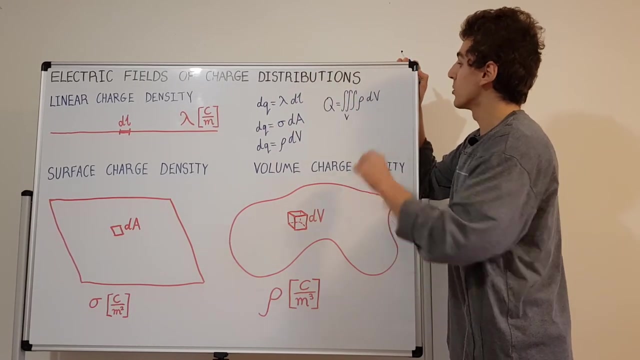 charge distribution. You can actually think of the charge density as a scalar field. There's no direction associated with any of the values, but every point in space has a scalar value. So what you can do is you can integrate the entire 3D space and what you will get is 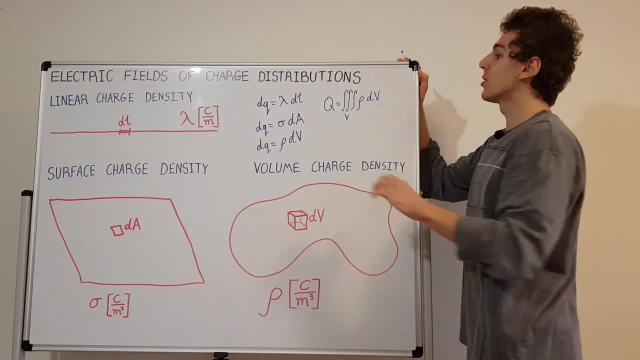 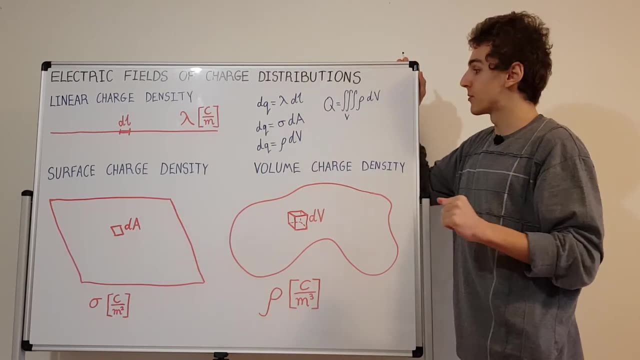 the total charge q. So how would we go from getting this tiny, infinitesimal charge to the electric field? Well, if you know from Coulomb's law, as we discussed before, you would integrate that and you would sum up over all of the charges. 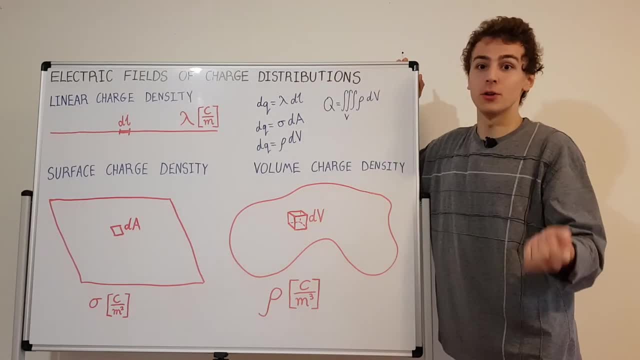 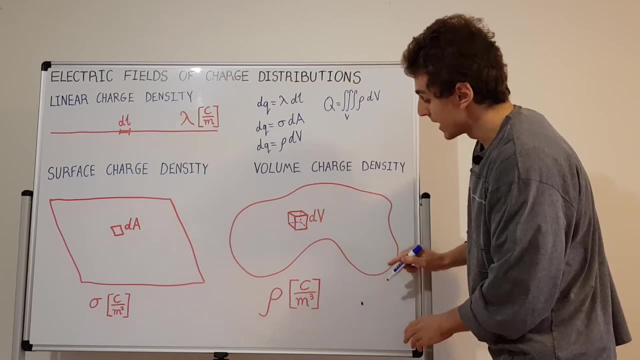 So the electric field would be the force per unit charge at any point, and so you would pick some point. So if we picked a point over here, what we'd have is a contribution from this little chunk right. There'd be a contribution from there. 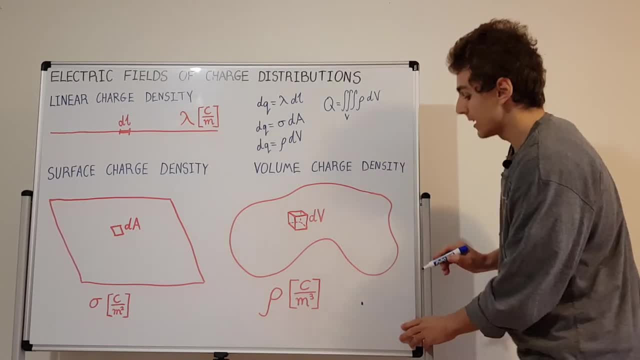 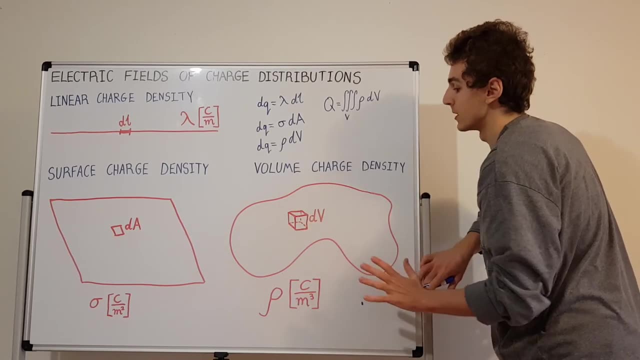 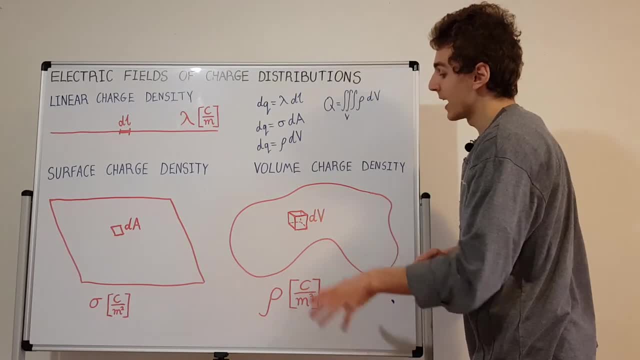 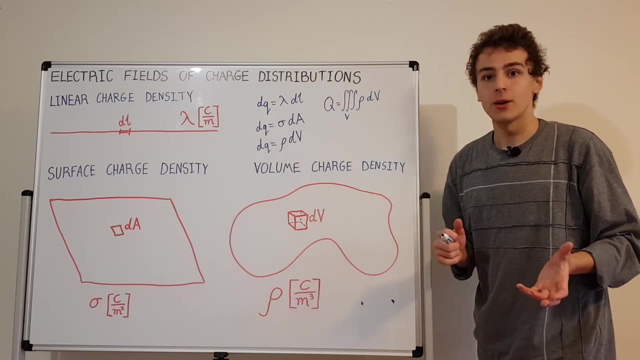 So Isaac Newton was actually dealing with these kinds of problems, and it took him a long time to actually rigorously define integration and to work it out in three dimensions. right, Because intuitively it seems like the electric field at this point has to be due to all of 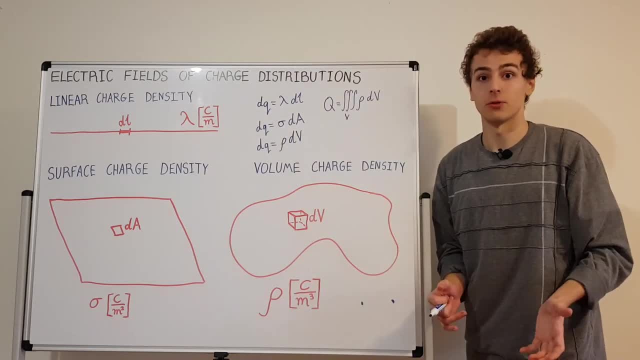 these charges. But how do you prove it? Well, you do the integral And it turns out it's a volatilization. It turns out it's a volume integral, It's a triple integral: dx, dy, dz, if it's in Cartesian coordinates. 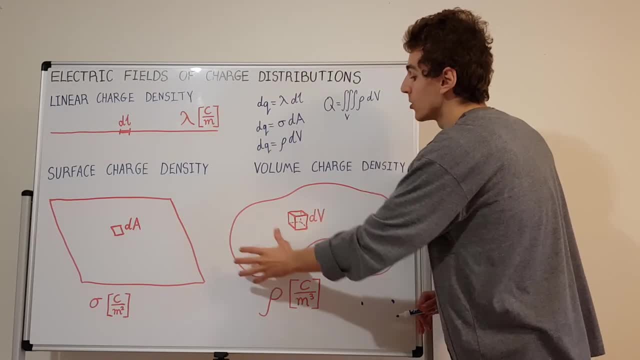 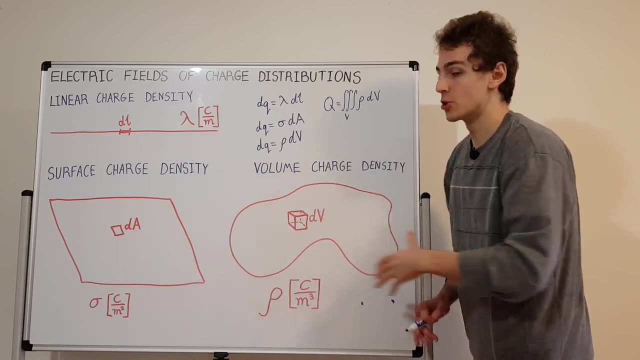 And you have to integrate all of this. take all the contributions of all of these tiny little infinitesimal charges, the dqs, and that's going to give you the entire contribution of charge, And so then you can apply Gauss's law for electric fields. 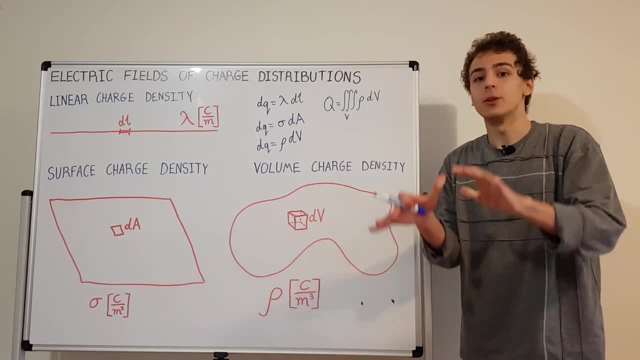 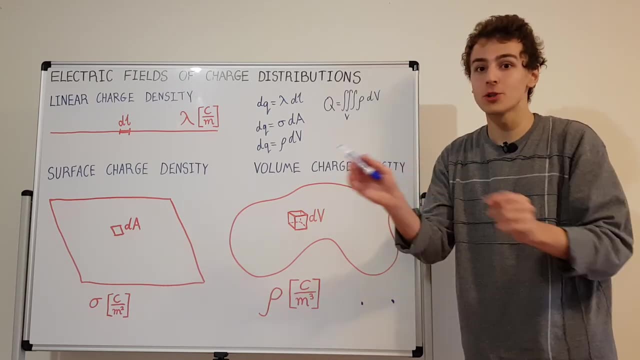 And Gauss's law for electric fields tells you that if you take a surface and you enclose a bunch of charge, right, It could be some kind of continuous charge distribution, It could be point charges. Those guys are going to produce an electric flux. 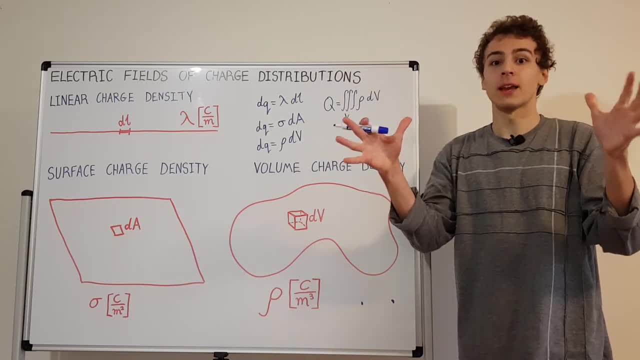 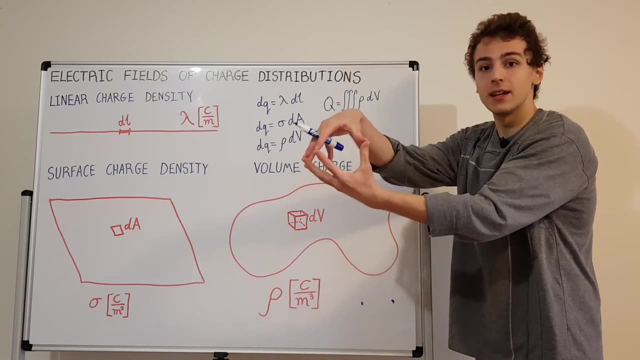 So there's going to be an electric field coming through the surface. If there's no charges inside that surface, there's not going to be any electric field. So if you have any, if you pick a surface in empty space and there's no charges there, 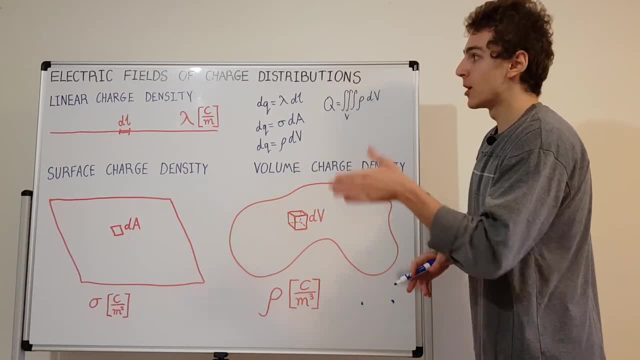 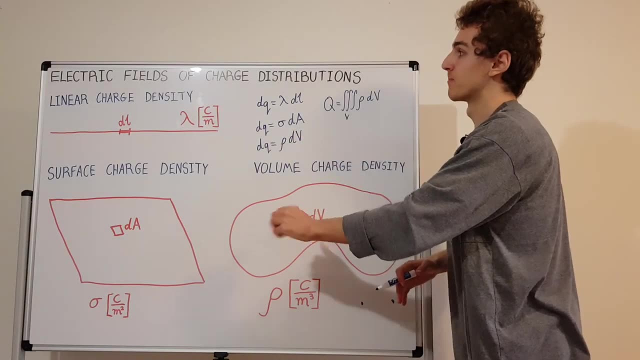 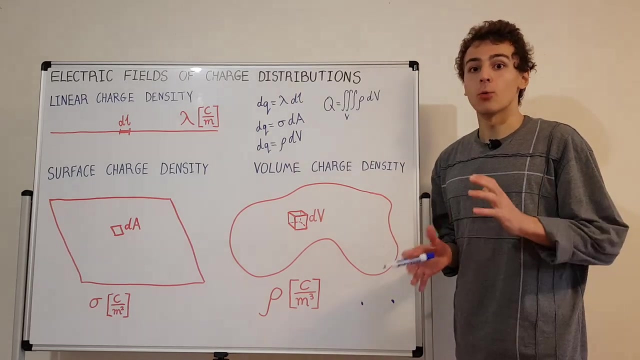 there's going to be no electric flux through that surface. So Gauss's law for electric fields is what you would use after you have figured out this, this kind of charge distribution. So this video has the aim of just giving you a brief overview of some of the charge density. 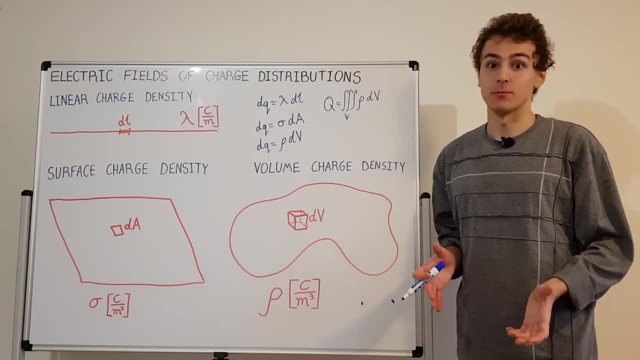 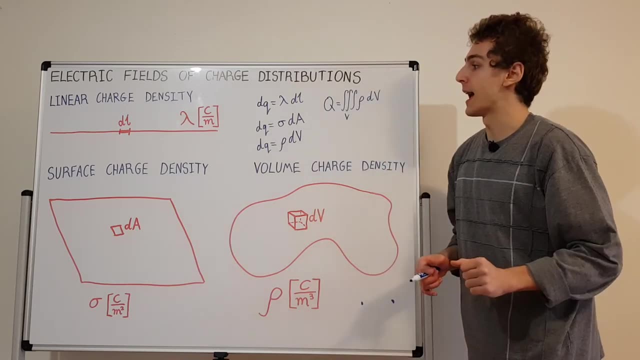 quantities that are very useful for electrostatics problems. So I hope this was helpful. This is some of the fundamentals of electrostatics and practice with some of these problems, and you'll find that it's going to become very intuitive and good luck with that. 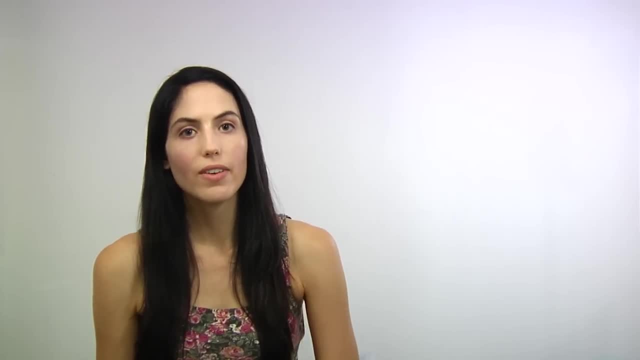 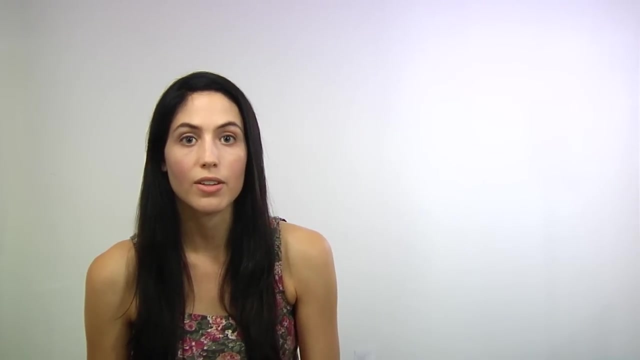 Hi guys, I'm Nancy and I'm going to show you how to find the domain of any function. The domain is kind of an annoying question that you'll get about a function, but it can be very simple And all it means is all possible x values that you can have in your function. 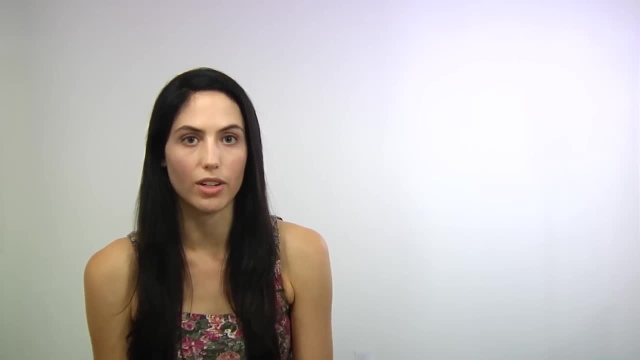 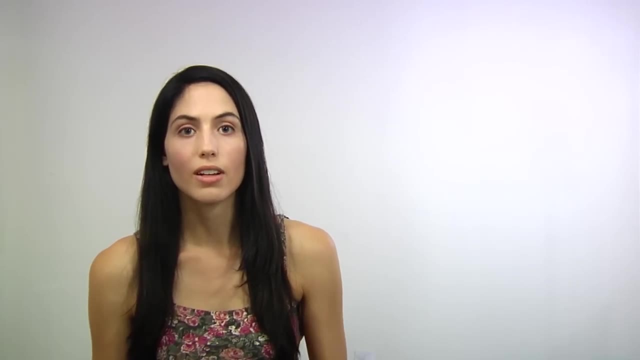 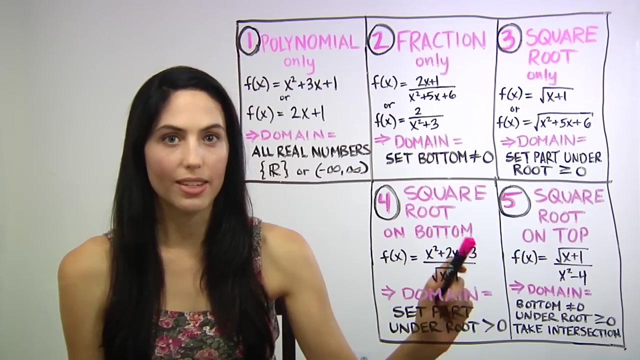 So all allowable x values that you can have in your function. To do this, you should already know how to solve a quadratic by factoring and how to solve an inequality. Okay, so these are the five types of functions you might have to find the domain for. I'm 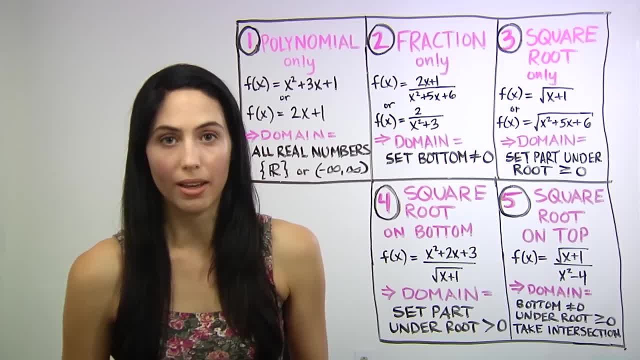 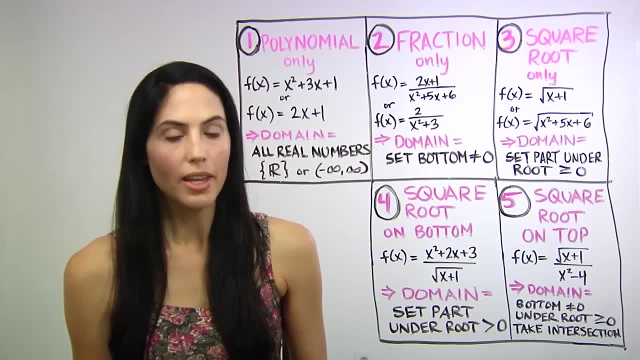 going to go through all of them. If you want to skip ahead, you can Just look down below in the description for the time. to skip to The first case is really easy If you have a polynomial, just an x expression like x.